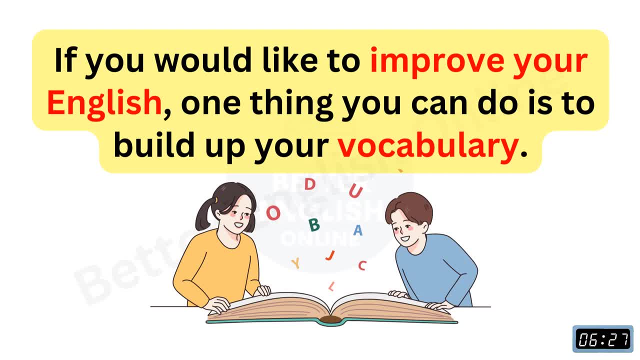 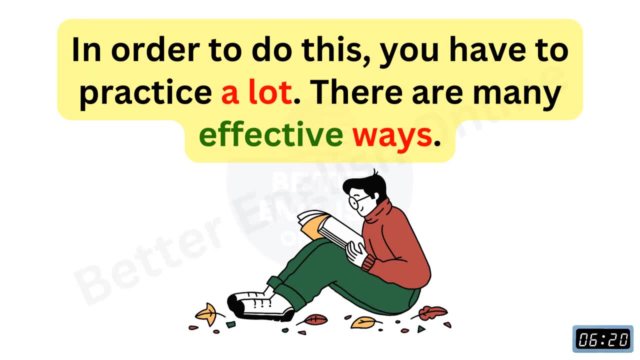 If you would like to improve your English, one thing you can do is to build up your vocabulary. In order to do this, you have to practice a lot. There are many effective ways. In order to do this, you have to practice a lot. 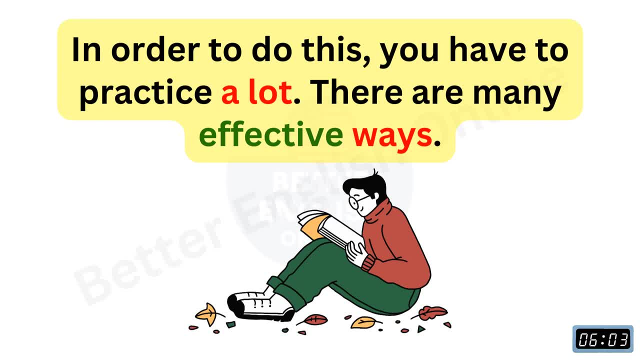 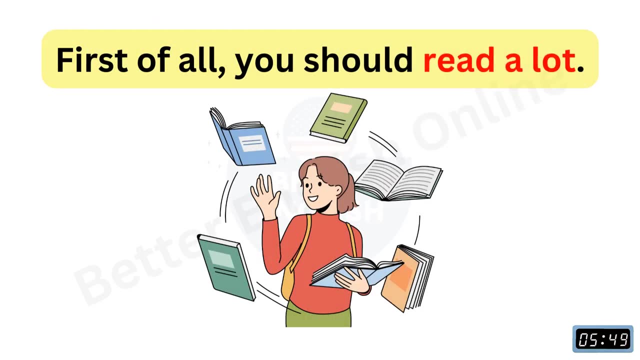 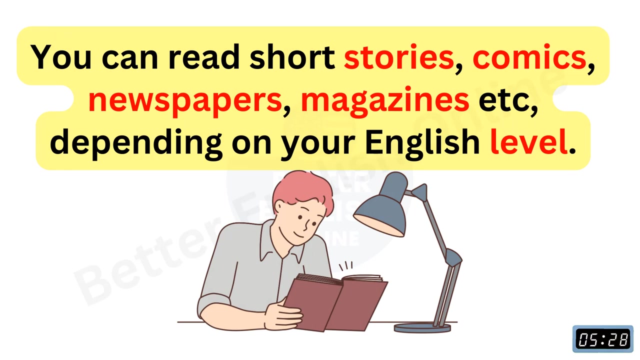 There are many effective ways. In order to do this, you have to practice a lot. There are many effective ways. First of all, you should read a lot. You can read short stories, comics, newspapers, magazines, etc. depending on your English level. 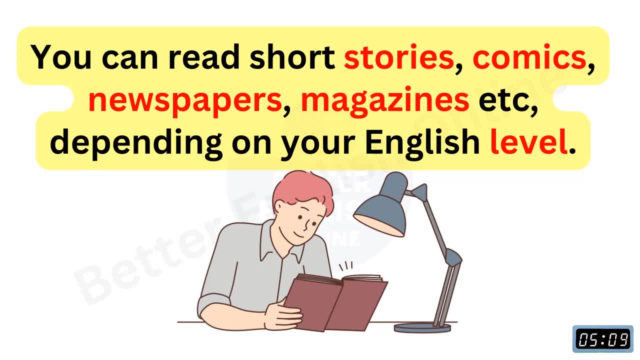 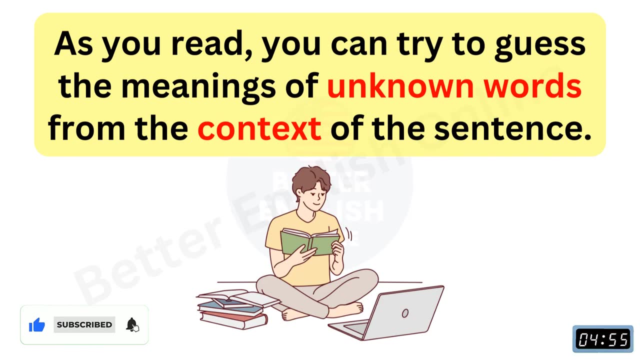 You can read short stories, comics, newspapers, magazines, etc. depending on your English level. depending on your English level, As you read, you can try to guess the meanings of unknown words from the context of the sentence. As you read, you can try to guess the meanings of unknown words from the context of the sentence. 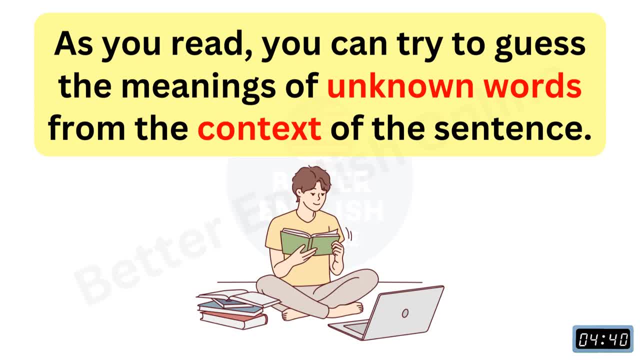 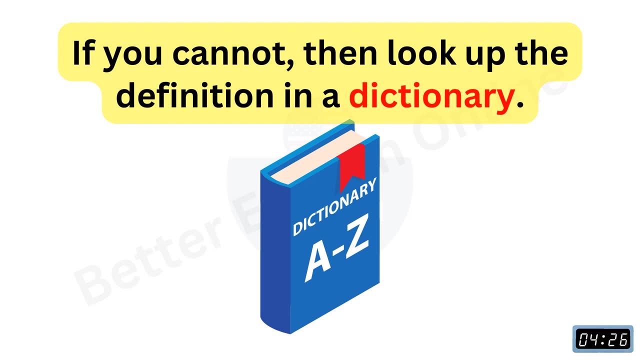 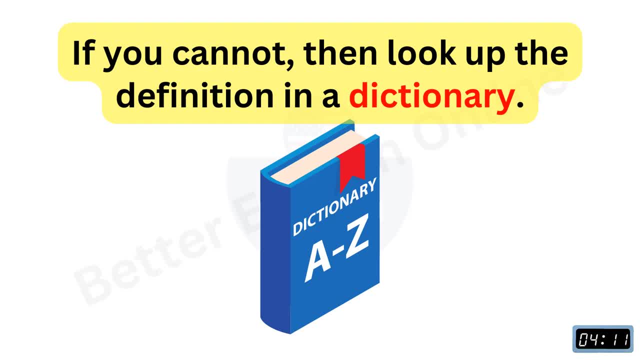 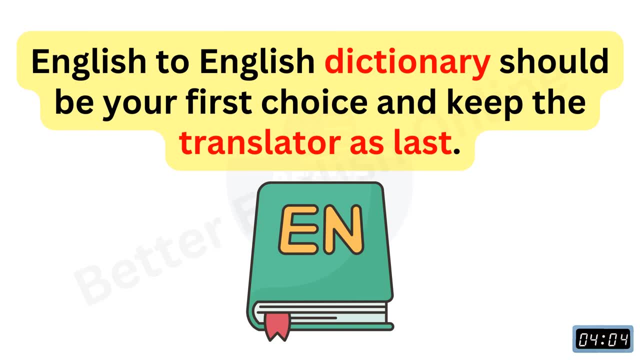 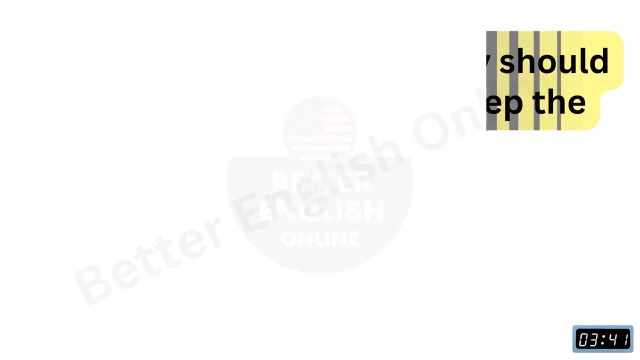 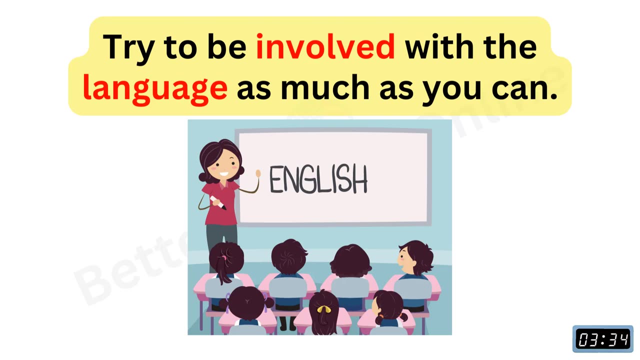 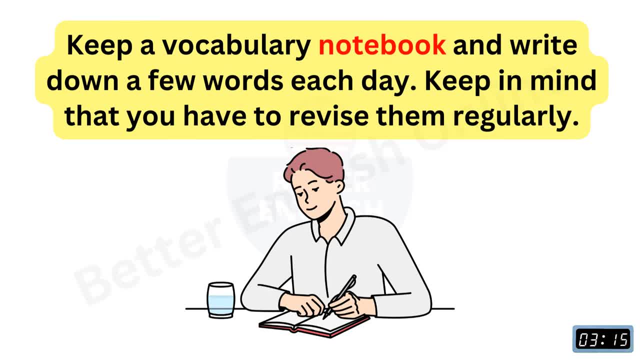 Keep a vocabulary notebook and write down a few words each day. Keep in mind that you have to revise them regularly. Keep a vocabulary notebook and write down a few words each day. Keep in mind that you have to revise them regularly. Keep a vocabulary notebook and write down a few words each day. 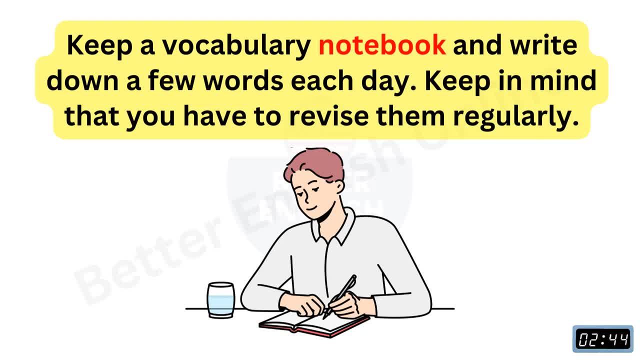 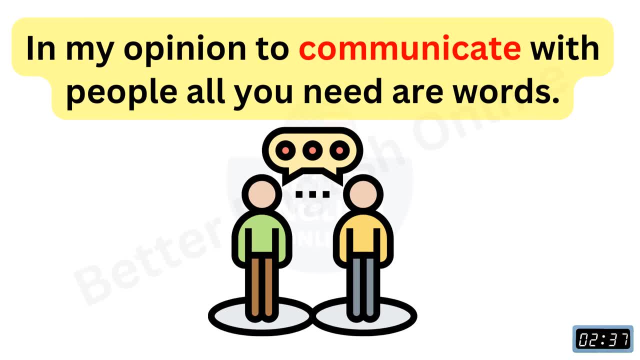 Keep in mind that you have to revise them regularly. In my opinion, to communicate with people, all you need are words. In my opinion, to communicate with people, all you need are words. In my opinion, to communicate with people, all you need are words. 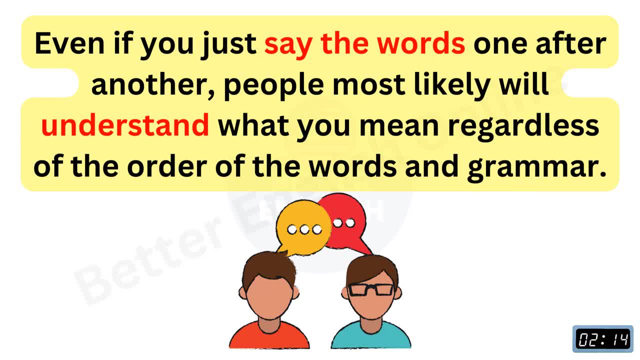 Even if you just say the words one after another, people most likely will understand what you mean, regardless of the order of the words and grammar. Even if you just say the words one after another, people most likely will understand what you mean, regardless of the order of the words and grammar. 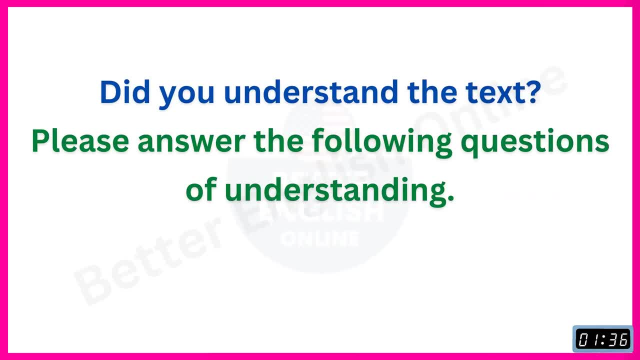 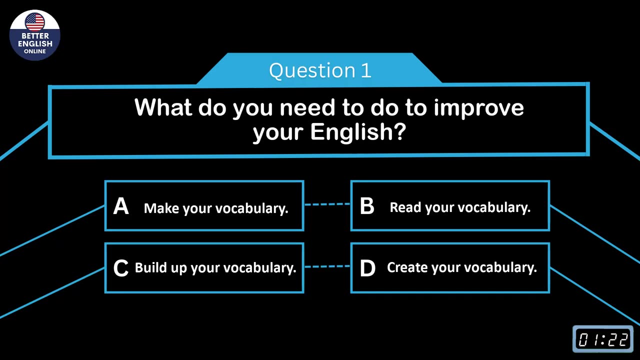 Did you understand the text? Please answer the following questions of understanding. Question number one: What do you need to do to improve your English? A- Make your vocabulary. B- Read your vocabulary. C- Build up your vocabulary. D- Create your vocabulary?